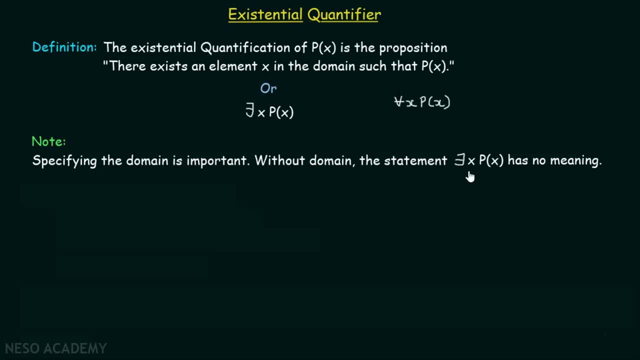 It should be well noted that if you didn't specify the domain, then this statement has no meaning. There are different ways to say there exists x- Px. You can say there is an x such that Px. You can say there is at least one x such that Px. 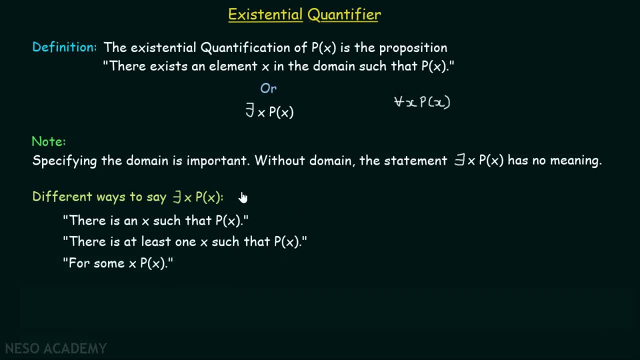 Or you can also say: for some x Px. These are the different ways in which you can say there exists x Px. Now here is one example I would like to discuss for cementing the concept of existential quantification: What is the truth value of? 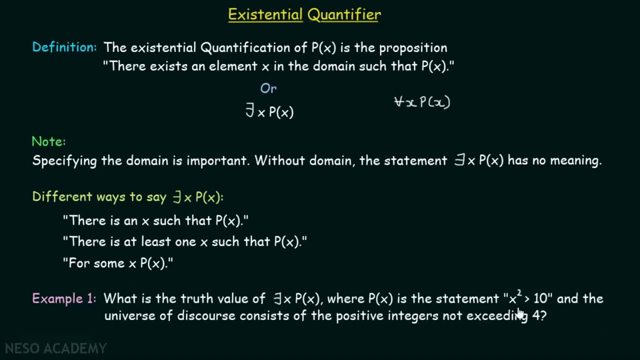 there exists x Px. where Px is the statement x square is greater than 10 and the universe of discourse consists of the positive integers not exceeding 4?. Understand this question carefully, that it is asking us to find the truth value of there exists x- Px. 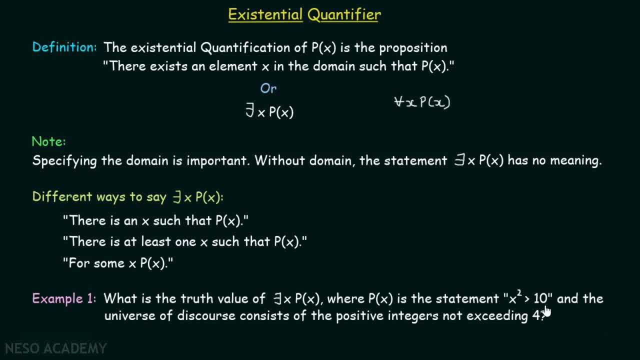 Px is the statement given to us. x square is greater than 10 and we have given the universe of discourse, or you can say, domain of discourse, consists of the positive integers not exceeding 4.. Now let me write the complete details over here. We know that. 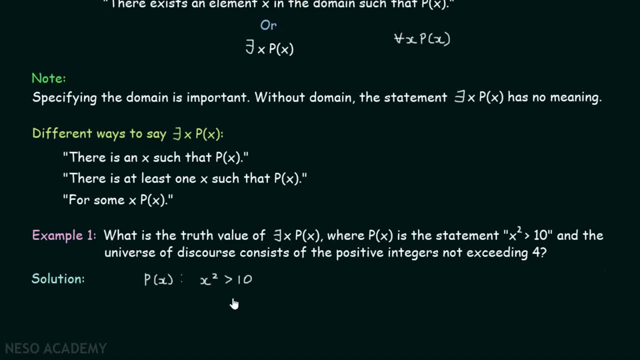 Px is the statement x square greater than 10.. Now if we replace this with x by 1, then we can say that this is 1 square greater than 10.. Please note the domain here. The domain consists of positive integers not exceeding 4.. 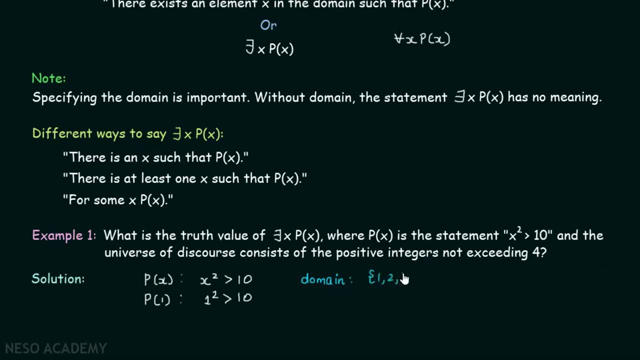 So let me write the domain here. The domain consists of all positive integers not exceeding 4.. This is the domain right: 1, 2, 3, 4.. You can see over here that with x equal to 1, 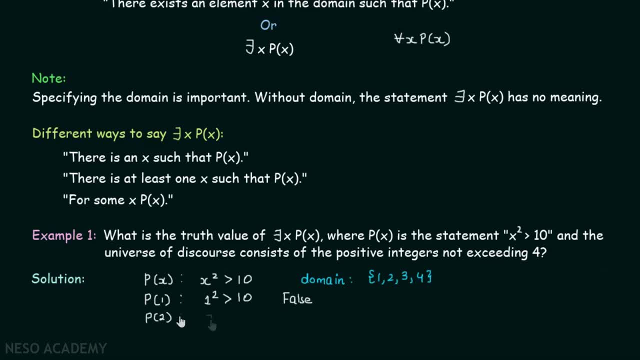 we are getting the truth value as false. Now, what happened in case of P2?? This will be 2 square greater than 10.. Obviously, this is also false Because 2 square is 4, 4 is not greater than 10.. 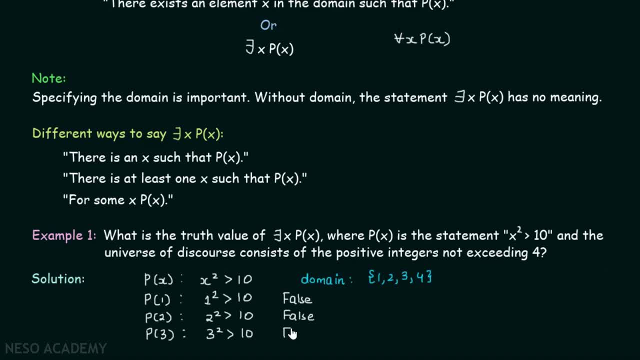 For P3, it will be 3 square greater than 10.. Still it is not greater than 10.. Hence, this is false. And in case of P4, this will be 4 square greater than 10, which is true. 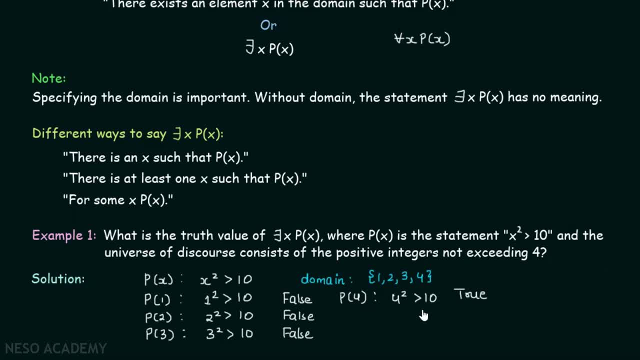 So obviously there is some x for which this statement becomes true. In other words, I can say that there exists x- Px is true, But please note that there exists x. Px means P1 or P2 or P3 or P4.. We know that P1 is false, P2 is false, P3 is false.